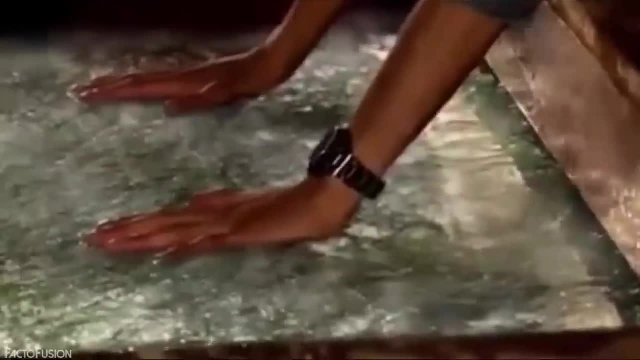 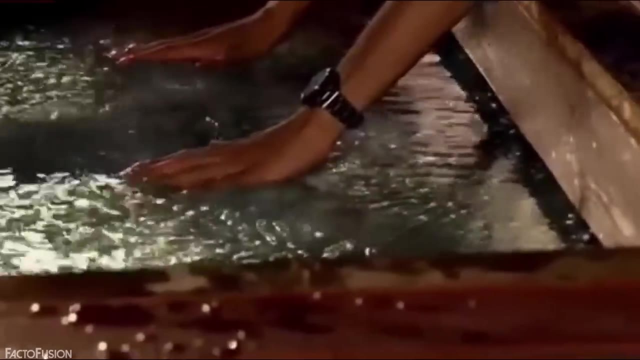 You might even be wondering as to how come he was able to do that. The trick is very much a planned trick of Dynamo, as usual. To begin with, he touches the water and the water starts to freeze into ice. But that did not actually happen, and here's the secret. 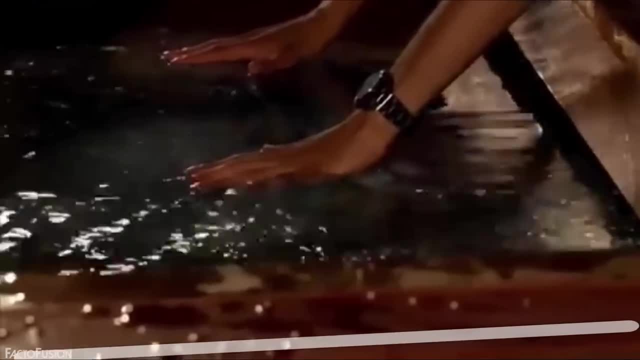 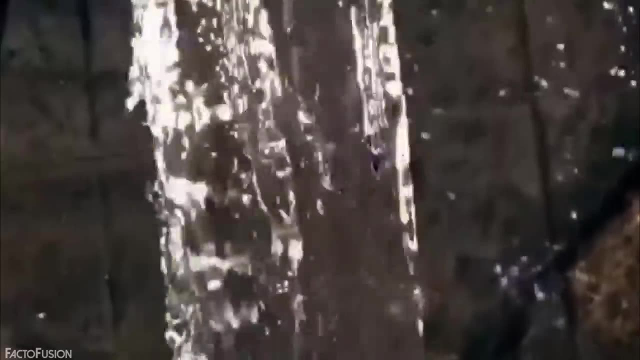 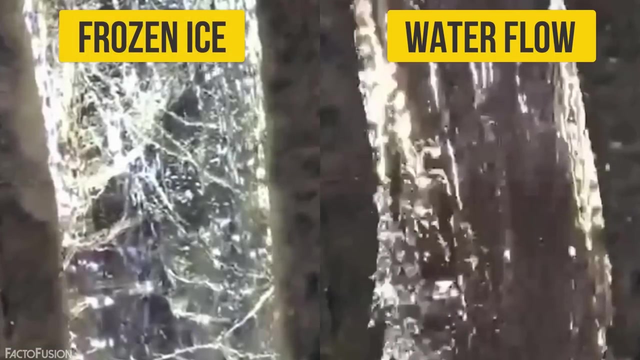 There was already a layer of ice at the bottom of the fountain water, which was made to rise above by pulling the water downwards, Also to amaze the audience. more so, Dynamo even froze the fountain water source. Well, if you look closely, the ice flow is actually narrower than the stream of water. 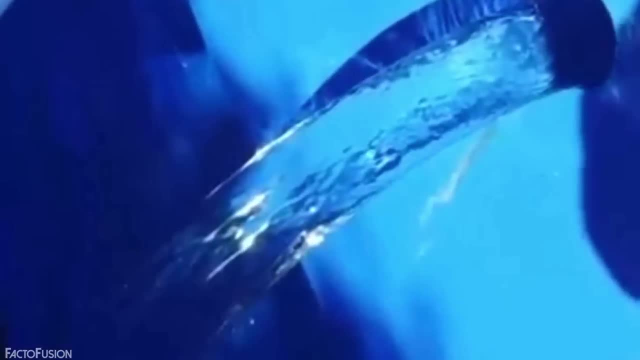 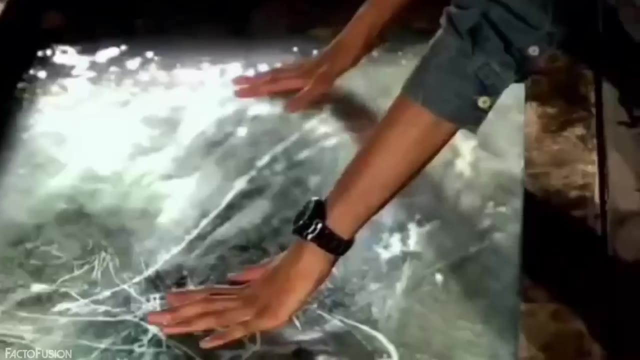 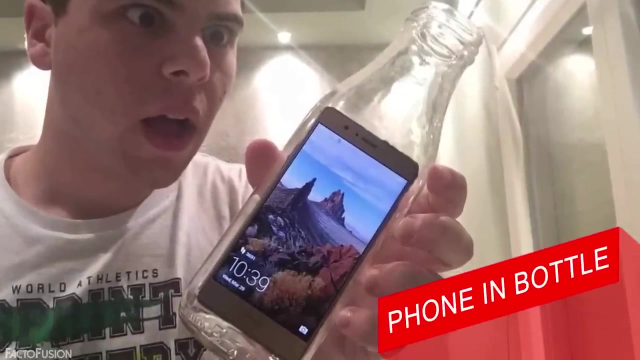 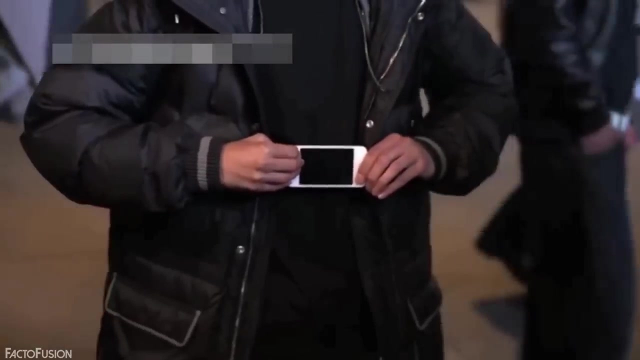 which makes it possible that the frozen stream of ice was already present and water was made to flow over it, Which was later stopped. that made it look like the stream of water was also frozen At number 6, Phone in a Bottle. Dynamo once performed a trick in which he takes an iPhone from a woman and in one quick moment turns it into a small phone. 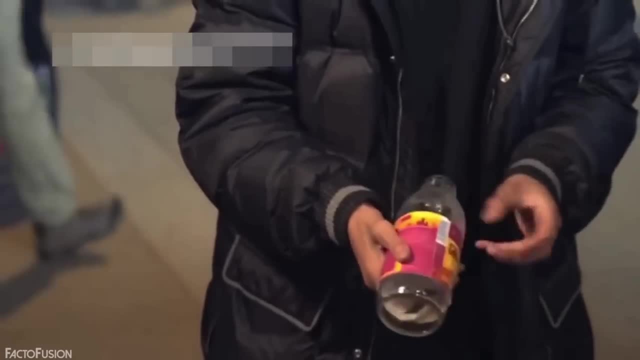 Then he takes a glass bottle from a man, puts that small phone in the bottle and here comes the final part of the trick: He converts that small phone back into the original bigger iPhone. He converts that small phone back into the original bigger iPhone. 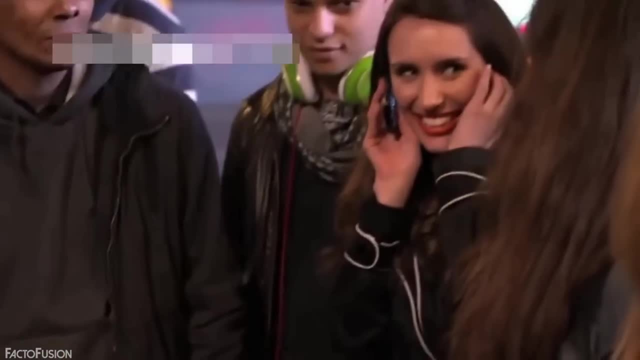 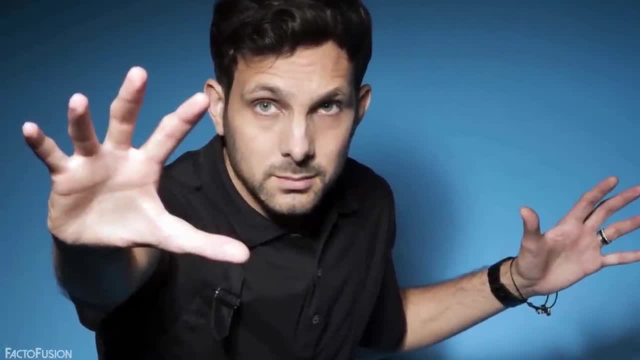 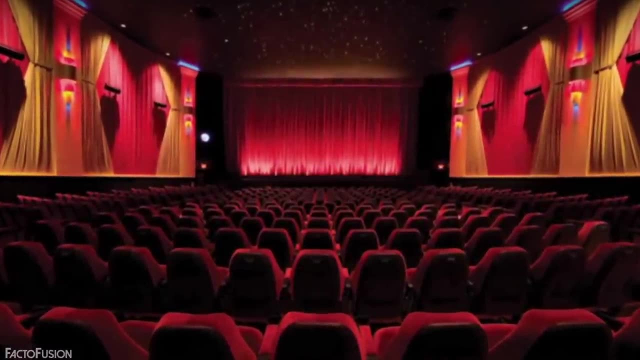 So how did Dynamo actually perform this trick? Well, here's the secret: Before this trick was performed, Dynamo had already taken the woman's iPhone- maybe during a previous trick or somewhere else- and gave her an identical copy of her iPhone. 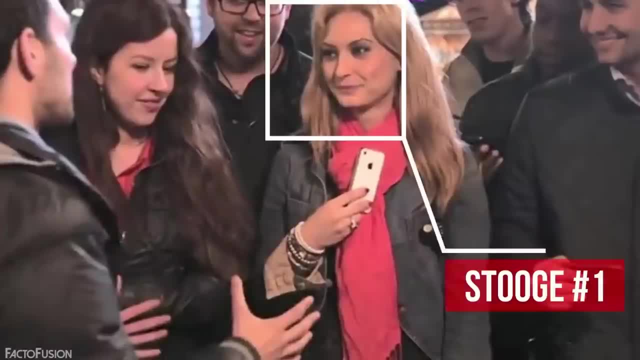 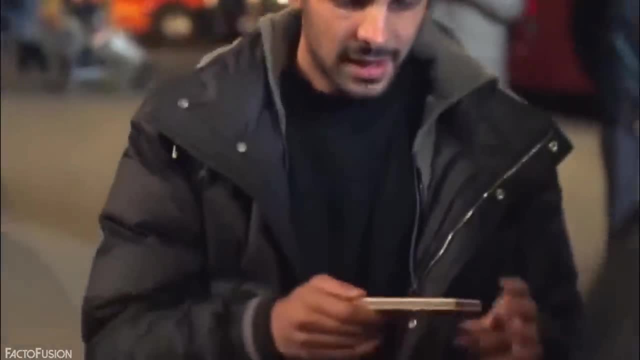 Then they started filming this trick, with the woman already holding a fake iPhone. So Dynamo takes her iPhone with the same iPhone. So Dynamo takes her iPhone with the same iPhone. So Dynamo takes her iPhone with the same iPhone. The 했어 thinks this is every girl's iPhone because its the most expensive iPhone on the market. 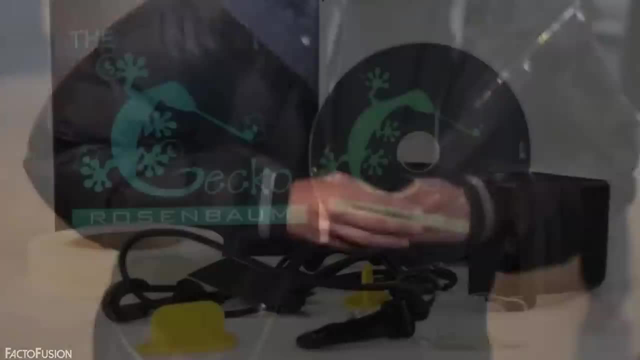 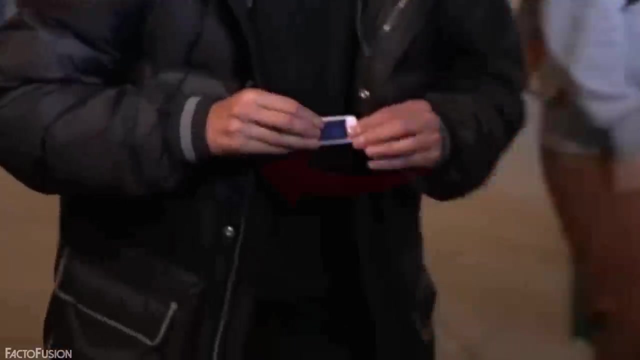 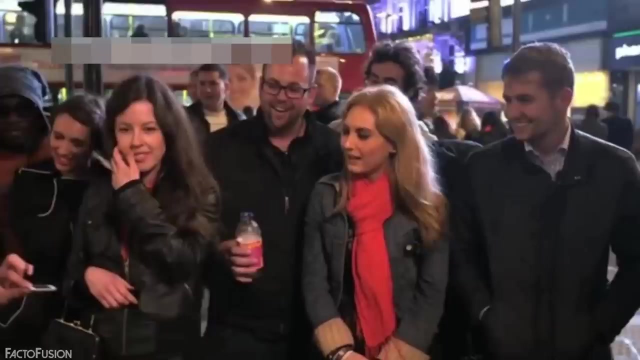 And now he can use hissky bands to make the necklace, just like the democracy or the. At the same time, he takes a smaller version of the phone from his left sleeve, which he had already prepared, and then fits this small phone into the empty being given by the man, who is also a stooge. 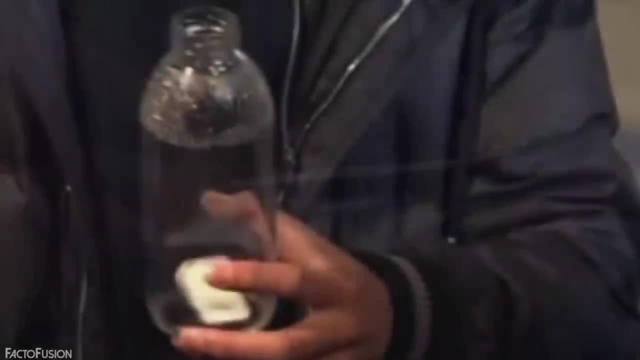 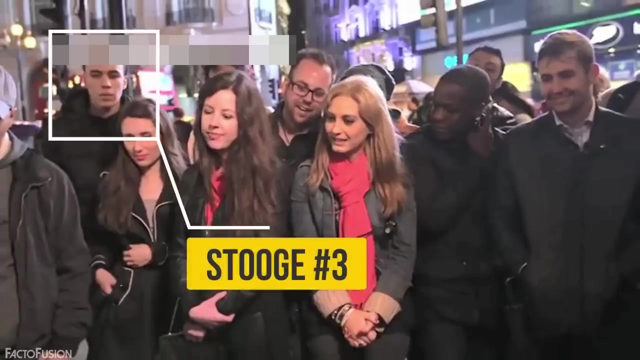 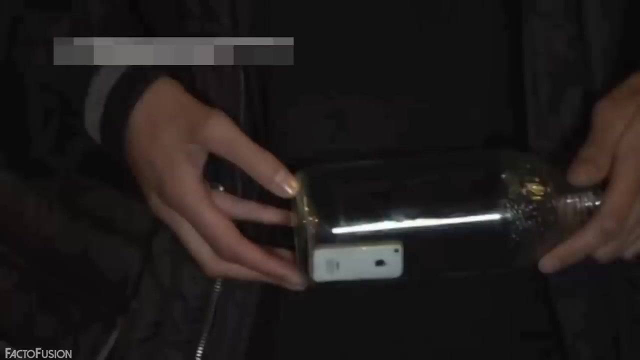 For the final part of the trick. the bottle you see now has been exchanged with the previous bottle And it was during this camera cut when the bottle was exchanged by the third stooge in this trick. Now this already prepared bottle has a black card which separates the replica of the small phone and the woman's original iPhone, which was taken before the trick. 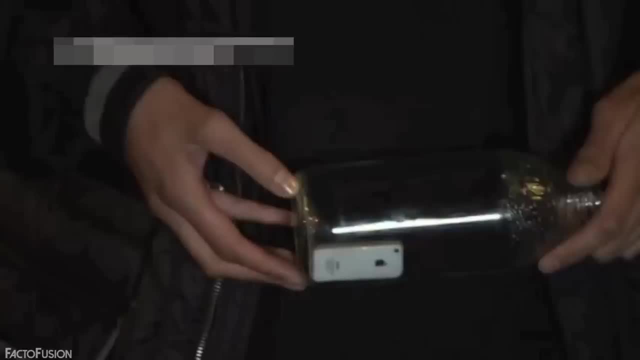 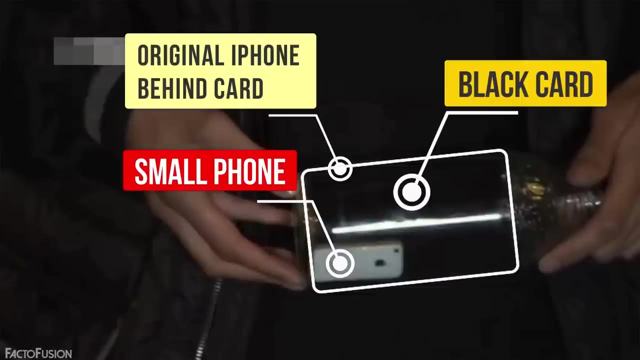 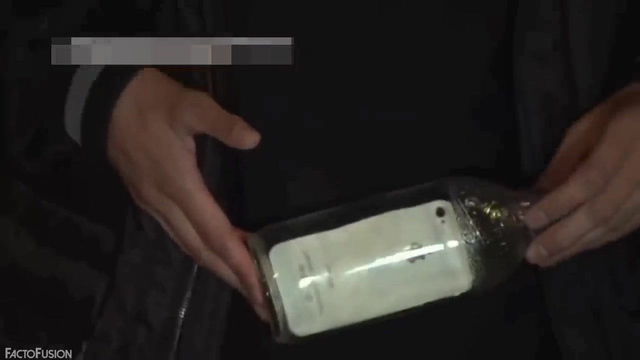 Here the iPhone is hidden behind the card which blends with Dynamo's black t-shirt. If we pause here, you can see the outline perfectly. Now, to convert the small phone back to the original iPhone, Dynamo just rotates the bottle and shows the original iPhone with the small phone hidden behind the card. 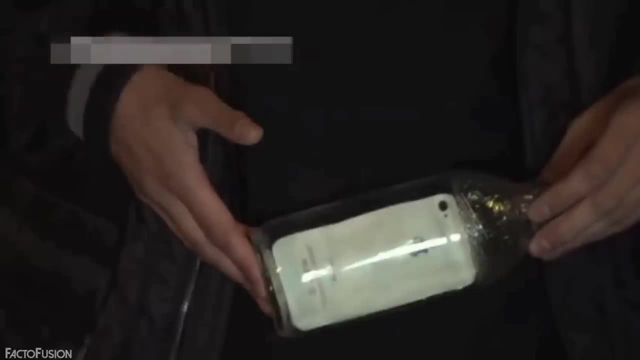 Here you can also see Dynamo's thumb going down, which confirms that he rotates the bottle. At the same time, he makes that black card and small phone disappear using the gecko technique explained earlier. He finally rotates the bottle and the small phone is hidden behind the card. 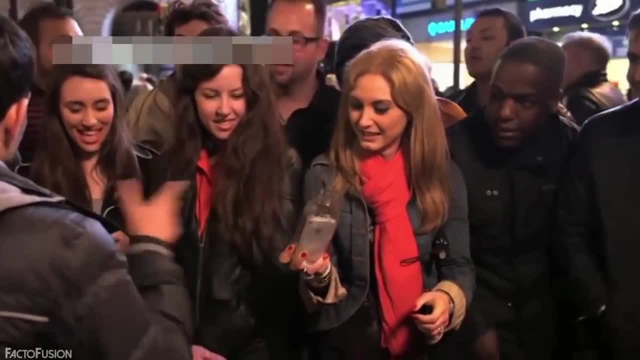 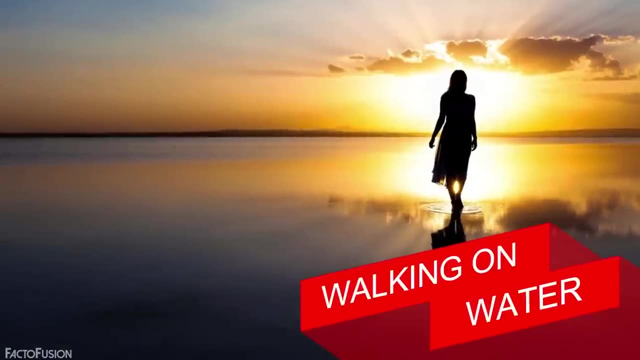 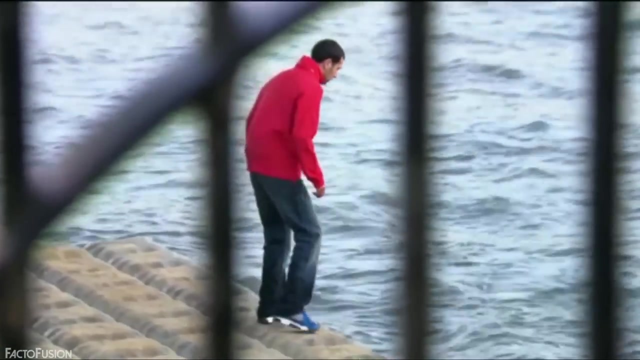 He returns the iPhone left in the bottle to that woman and of course it rings when her friend calls, because it is indeed her original iPhone At number 5, walking on water. You all must have seen Dynamo's famous video where he was seen walking on the water of the Thames River. 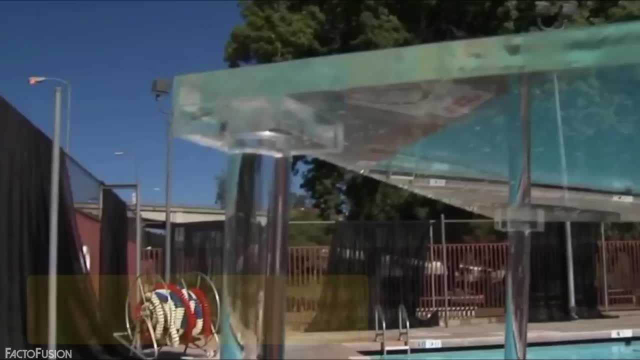 But how did he do it? Well, the answer surely lies in the plexiglass. Plexiglass, when submerged into water, is a very important part of the body, And when submerged into water it is almost hard to find. 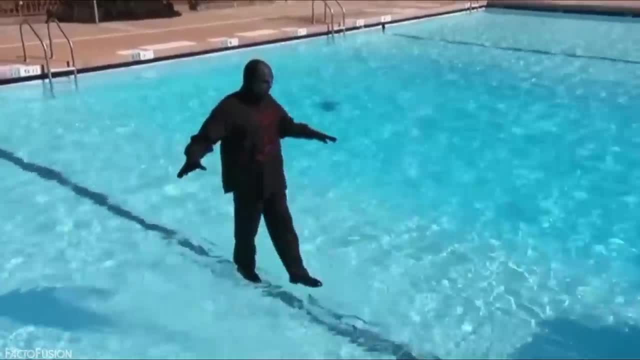 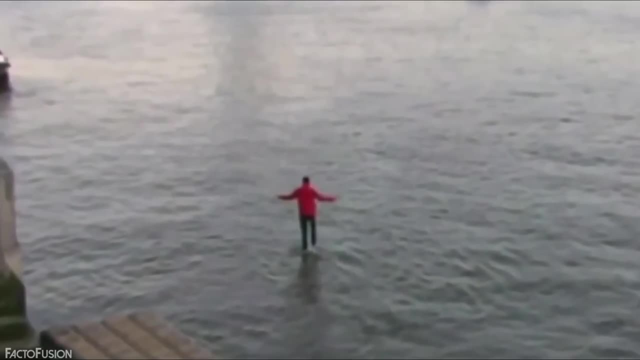 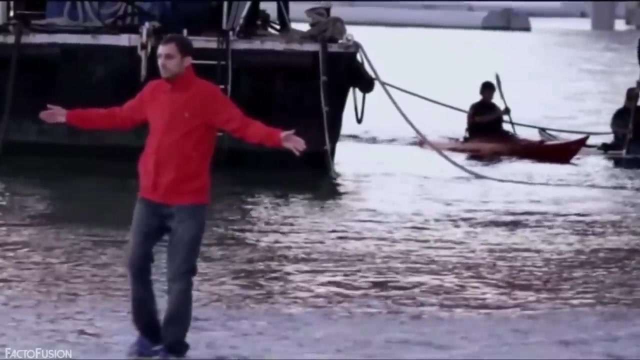 Because the density of plexiglass is almost like water. Plexiglass are clearly supported by plexi-tubes, and many magicians have tried the same variant in swimming pools and water lakes, No matter where it's performed, the answer, surely and always, is plexi-tubes and plexiglass. 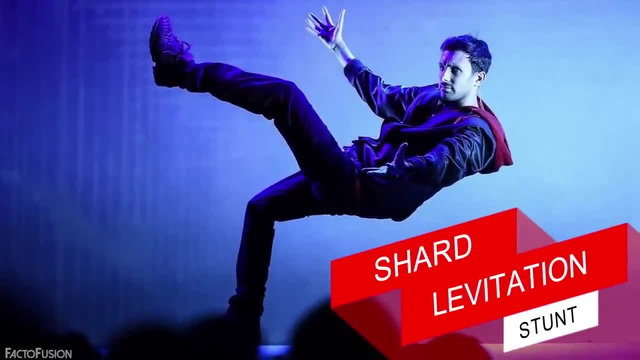 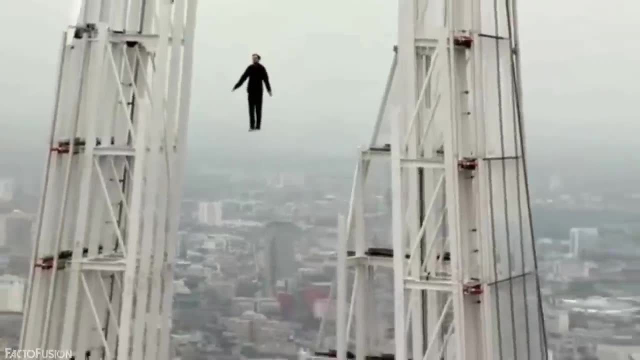 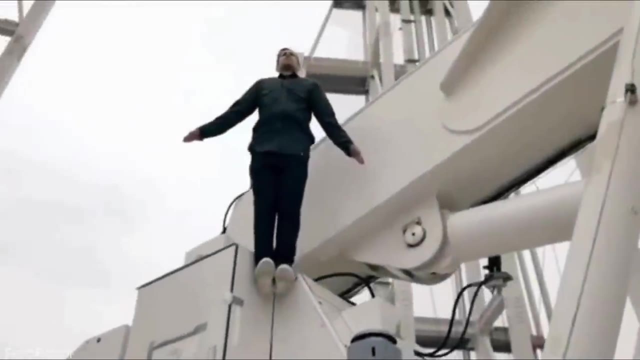 At number 4, shard levitation stunt Dynamo performed one of the greatest levitation actions ever performed by any other magician of levitating 1016 feet above the streets of london at the top of the shard. but if we take a closer look at what actually happened while filming this trick, 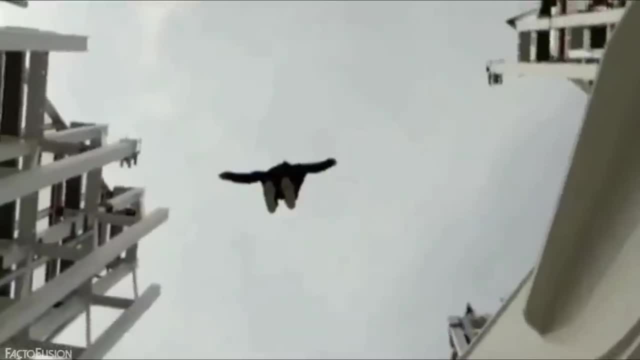 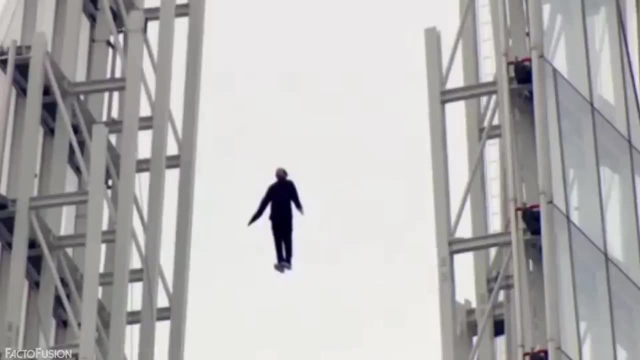 then it's not a magic trick but a clear result of filming and photography. the set was already prepared to film this trick, with cables attached to dynamo to pull him upwards and make the sense of levitation to the audience. dynamo stood in a mysterious position, seeming to gather his 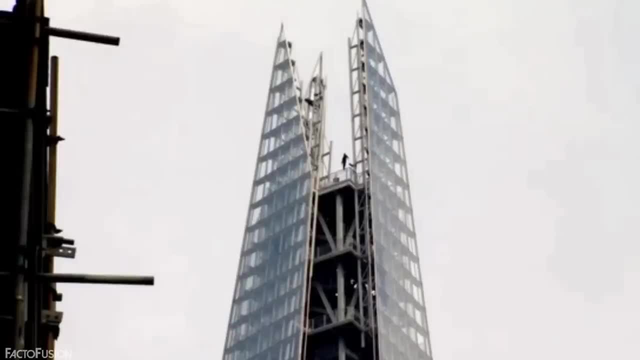 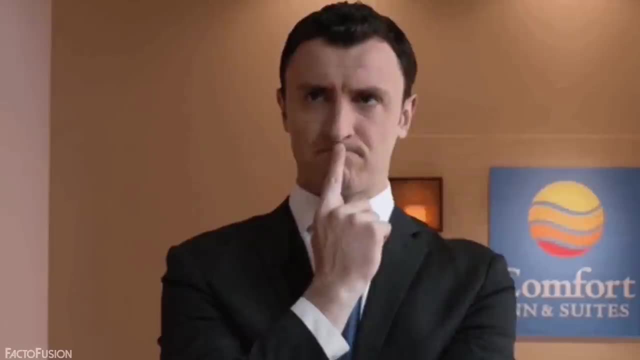 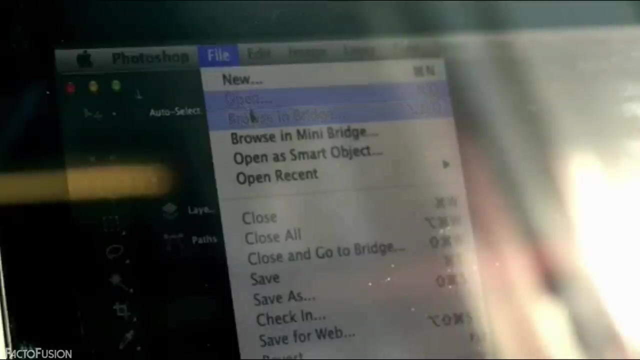 supernatural powers. he was then lifted in the air using cables attached to him and finally making him to levitate in between the clouds. an obvious question that might strike your mind is that: where are the cables in this video? the video, before being aired, had went through complete. 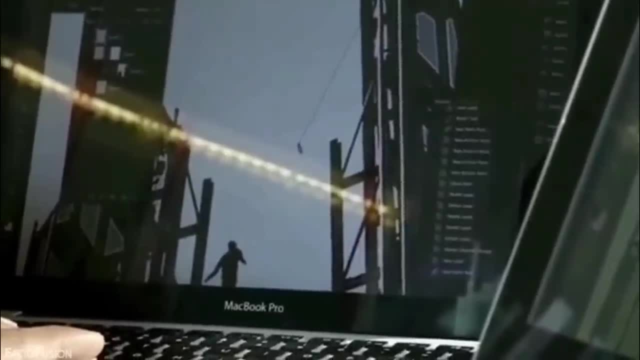 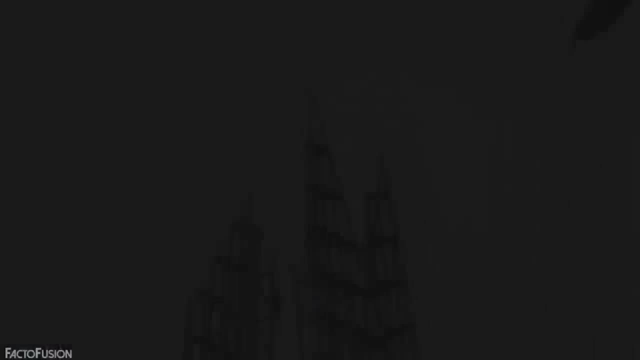 color correction and editing which hides the cables and gets them merged into the background. here's the comparison of the actual image and the image after editing. the entire trick was shot from a helicopter hanging up in the air above dynamo through various camera angles to avoid the cables. 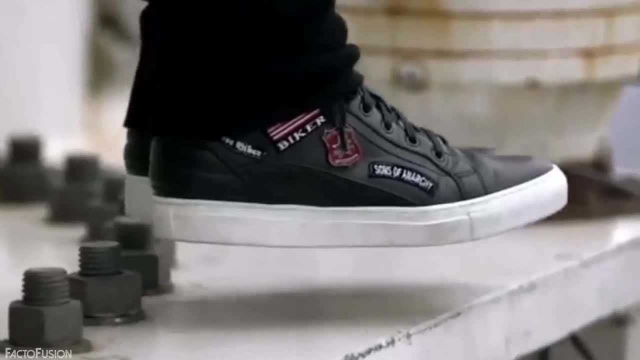 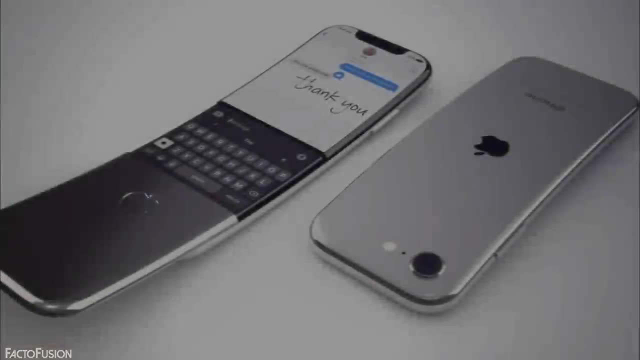 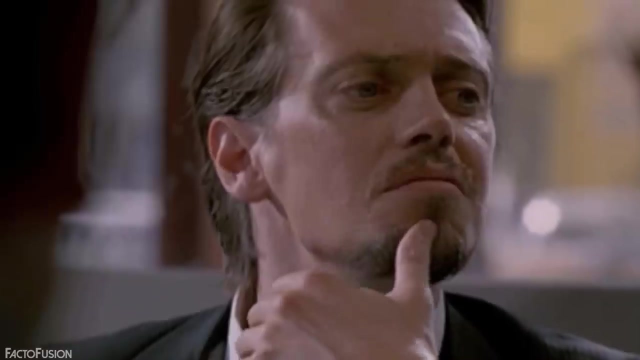 appearing in the video. so this makes it clear that there is no more magic to levitate in the air. but hats off to dynamo, who made it look real at number three: twisting an iphone. have you ever tried to twist your iphone from its center? obviously not, but dynamo has done it. 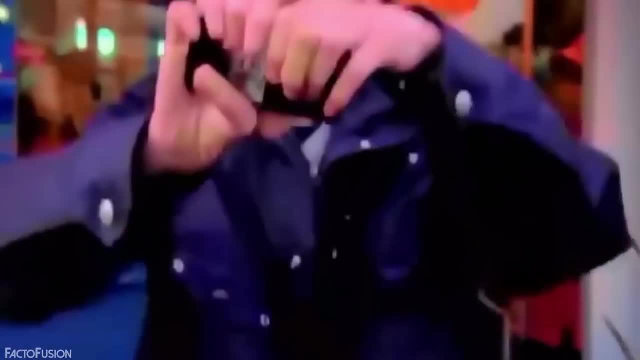 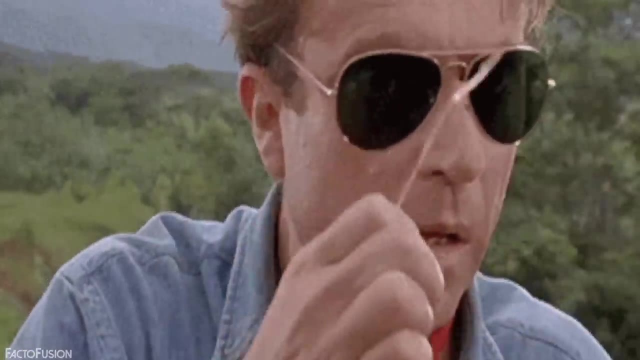 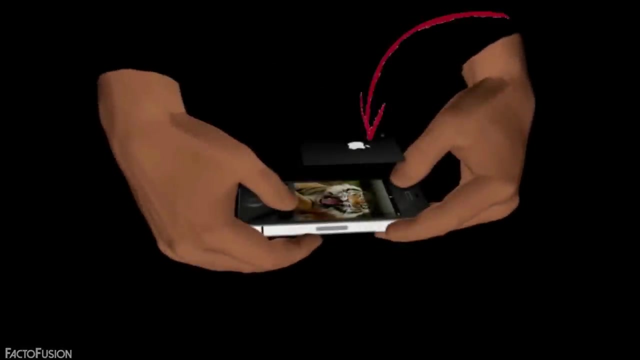 in front of people on the streets. he took an iphone and magically twisted it from its center to half screen and half back position. that's insane. but how did he do it? well, here's the actual trick. behind it, dynamo took an exact half back cover of iphone and placed it carefully. 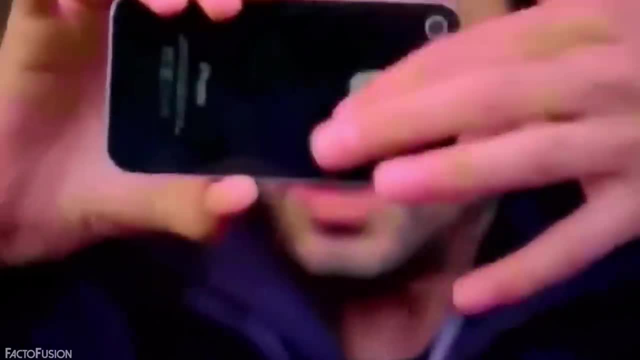 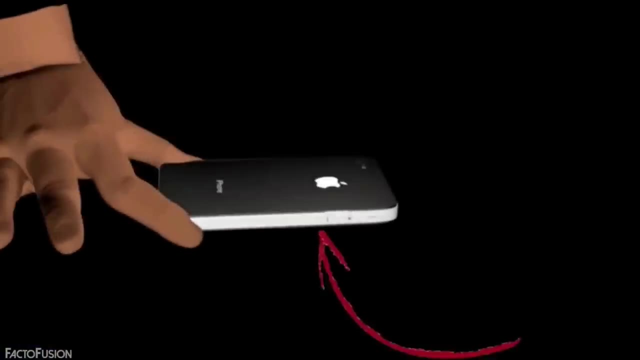 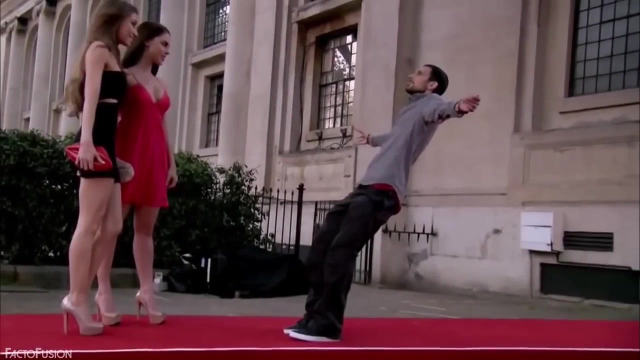 holding over the screen now showing his audience the back of the iphone. at first he covered the iphone with both of his hands and instead of twisting it, he just rotated the iphone entirely to the screen side with the half back cover placed over it. so want to impress someone like dynamo, watch this video till the end. screen with a link to the video. 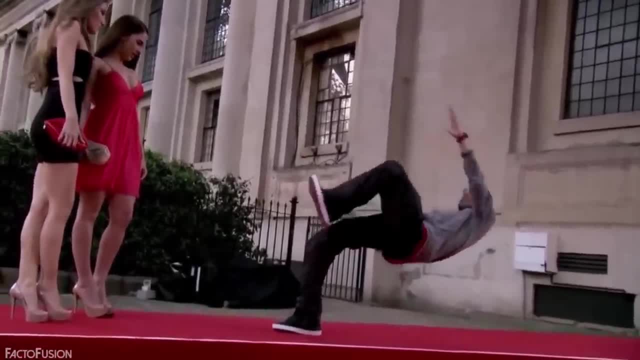 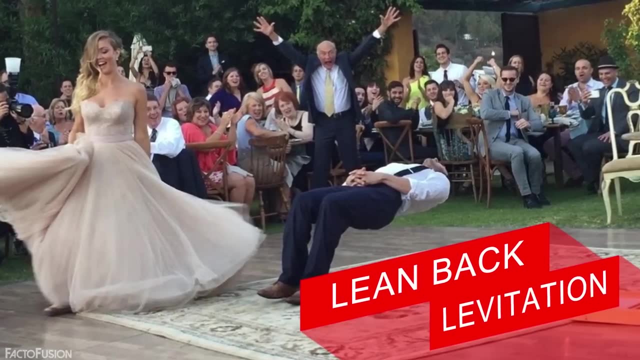 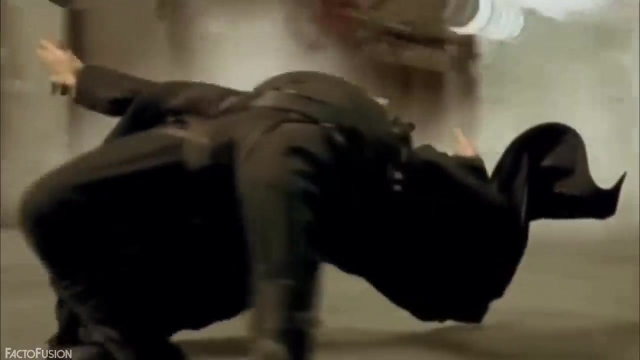 where you'll learn some easy to perform magic tricks to impress anyone you want, especially girls. at number two lean back: levitation. we all remember the iconic matrix scene, which was quite incredible. here you can see dynamo, the famous magician, who is performing this amazing trick with quite ease. 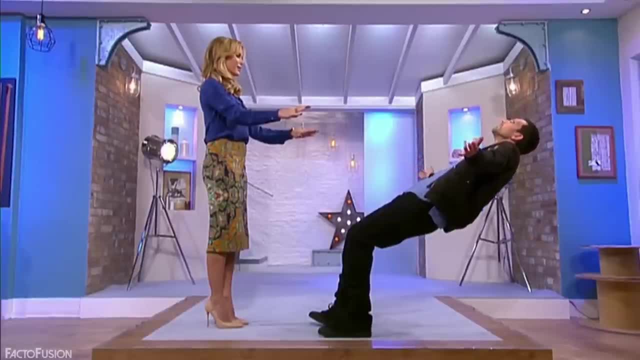 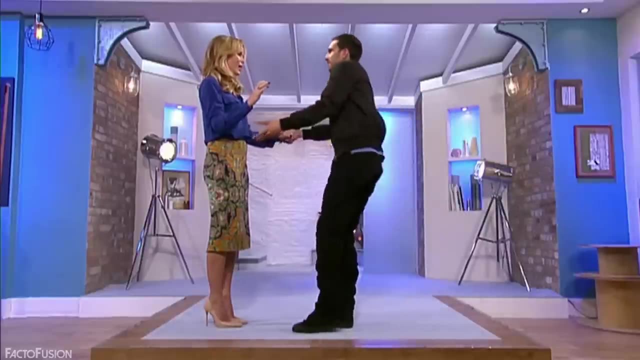 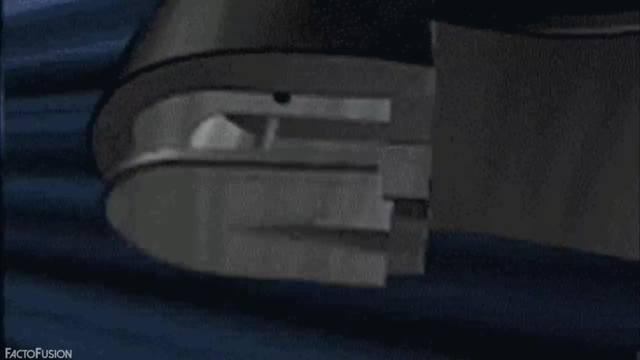 He leans back slowly till his body becomes parallel to the surface. Then he raises his left leg in the air and then all of a sudden gets back up without any problem. Ever wondered how Dynamo performed this gravity-defying trick? Well, here's the secret, And it's all hidden in the specially designed shoe, which has a heel that locks into pegs on the floor. 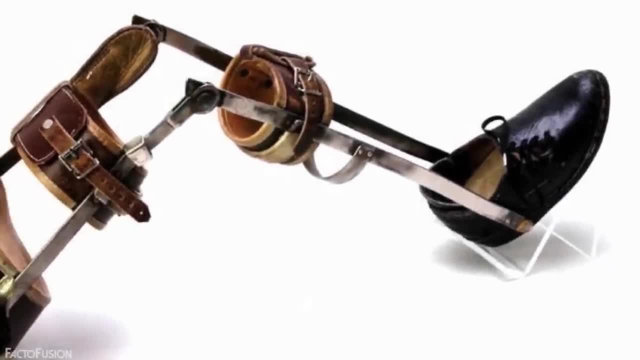 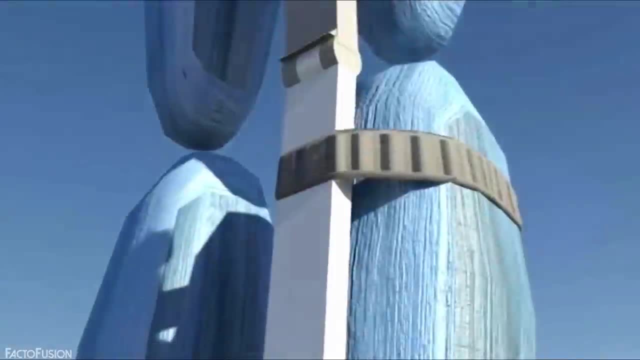 To support his full leg. the heel is connected to the steel-framed dual leg brace that locks out when he is just about parallel to the surface. This locking mechanism, combined with the heel mechanism, supports his body weight and shifts his center of gravity away from his upper body. 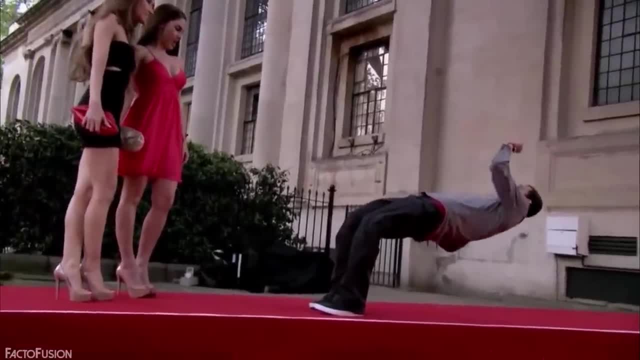 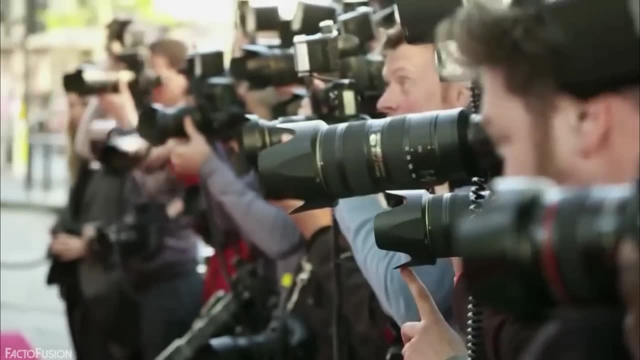 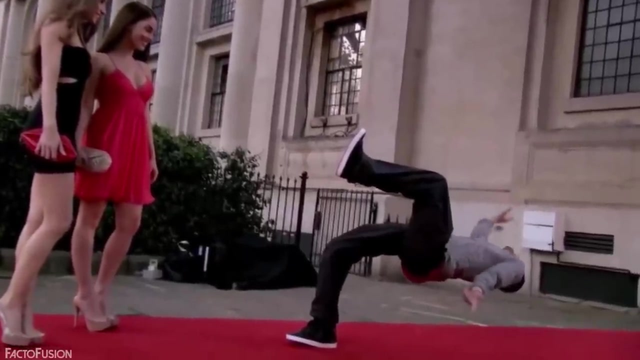 This allows him to stay balanced while leaning backwards at an impossible angle. Once he feels him being supported and balanced by his right leg, he lets everyone know that he's suspended in mid-air and slowly lifts his left leg. The interesting part here is that when Dynamo lifts his leg straight, 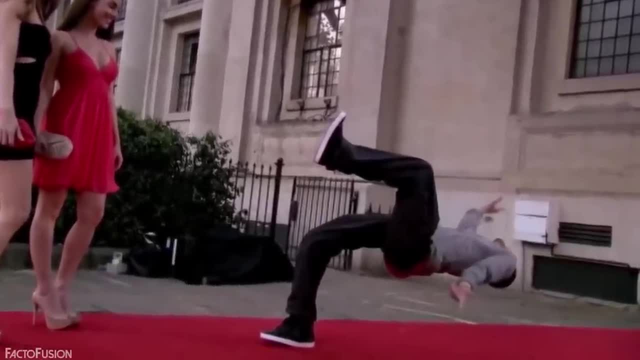 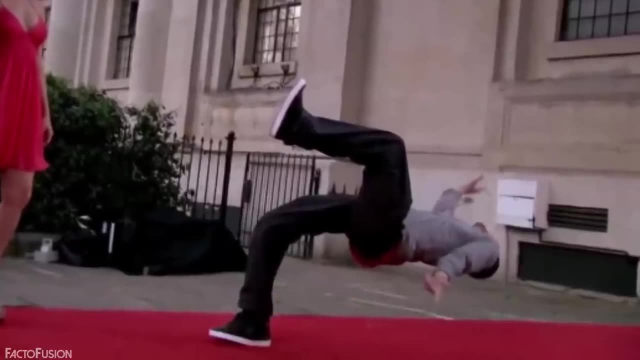 out of the air. he can't lift his left leg. It actually helps him balance by shifting his center of gravity even further towards his legs. In this trick, he also makes sure that his pants are long enough to prevent any exposure of the steel framework attached to his leg. 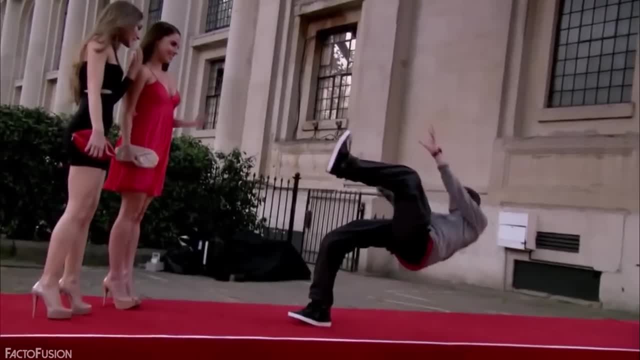 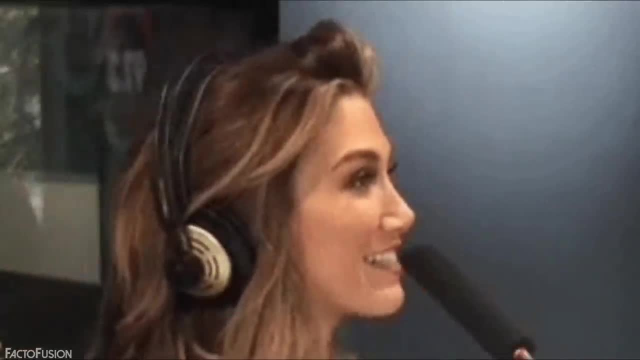 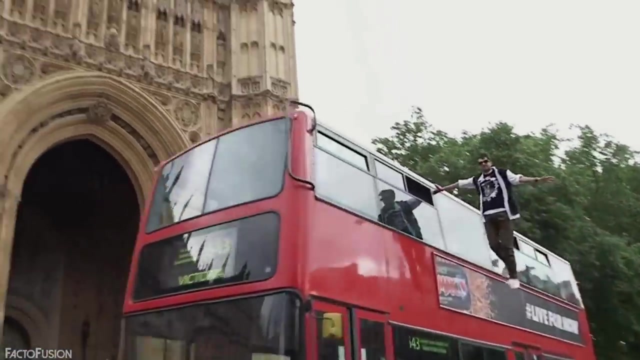 After impressing the girls with this matrix stunt, he slowly and steadily gets up. So finally, the number one trick on our list: Bus levitation trick. In this trick, Dynamo appears to be flying through the busy streets of London next to a double-decker bus. 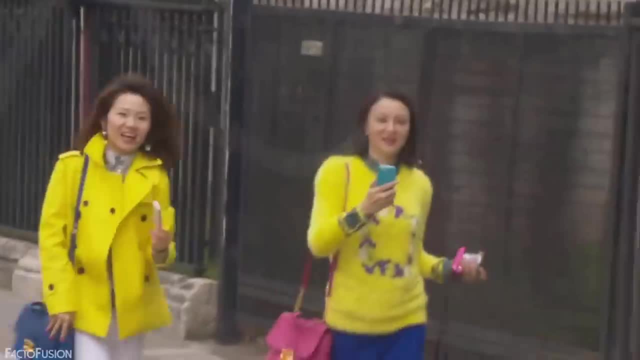 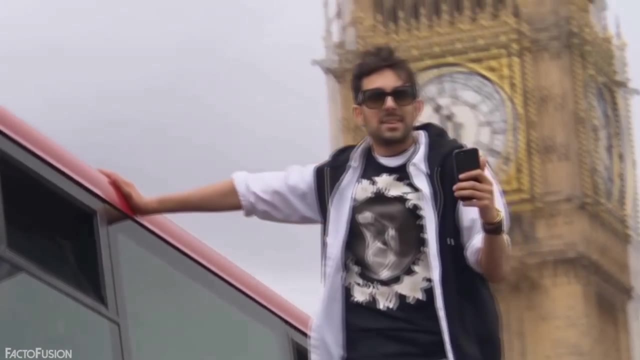 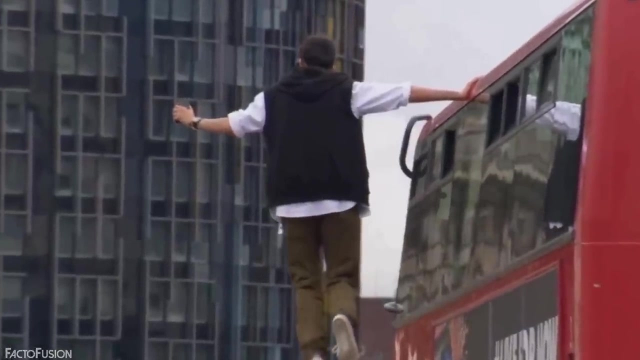 In this well-known trick, Dynamo stuns hundreds of spectators walking around as they watch him levitating with one of his arms holding onto the bus. So how did Dynamo manage to pull off this amazing feat? The secret here is quite simple and obvious once you pause and notice how his right arm 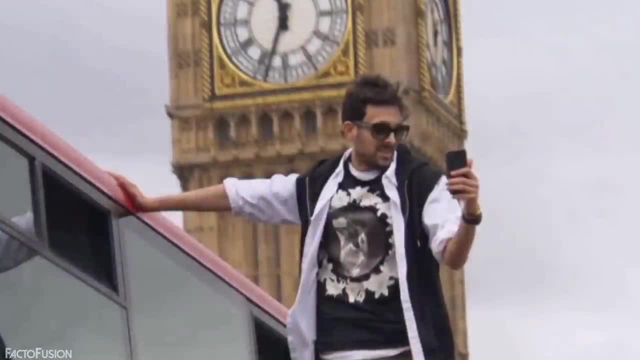 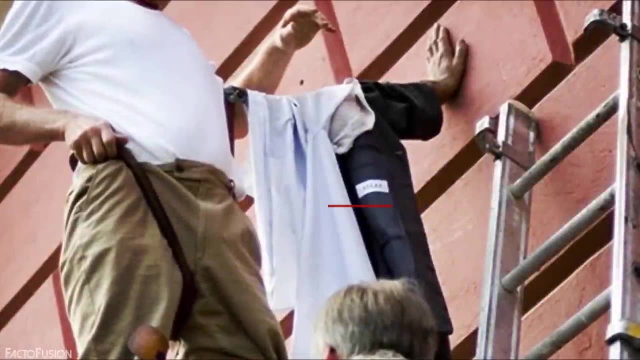 holding onto the bus never moves, not even vibrates or bends even slightly. This implies he uses a fake arm, And it isn't really his arm, because his so-called right arm is actually a firm metal rod attached to the bus and disguised as an arm. 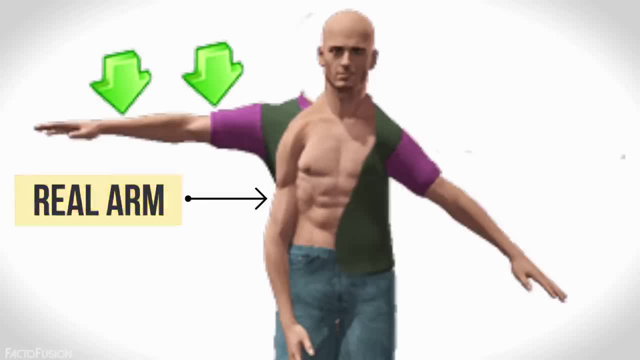 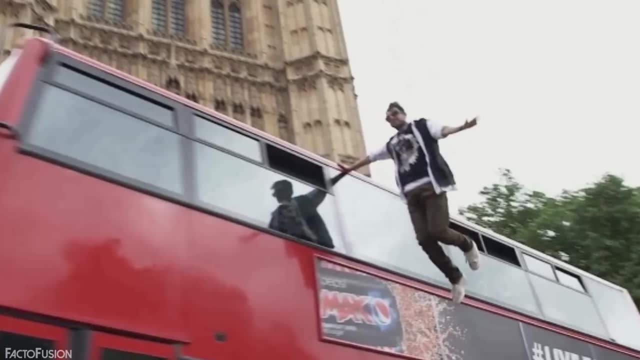 While his real arm is hidden under his clothes, squeezed tightly against his body. To support his body, he even wears a harness which is connected to the metal rod, and that is how he stays in the air. To make the illusion look even more convincing to the viewers, his legs and his left hand. 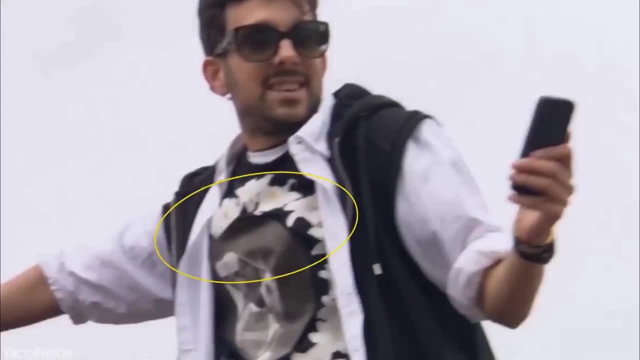 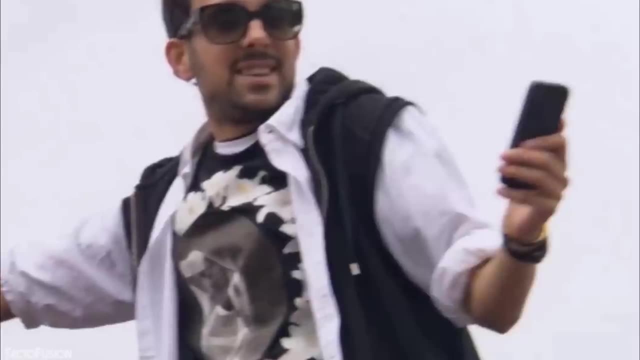 are free to move around easily. You can even notice the bump in his shirt that looks like an arm, but it's not an arm, it's a leg. It's an arm around his front. He intentionally wore this artistic shirt to hide the bump. It also explains why he uses a phone in his other arm, and that is to move and divert.